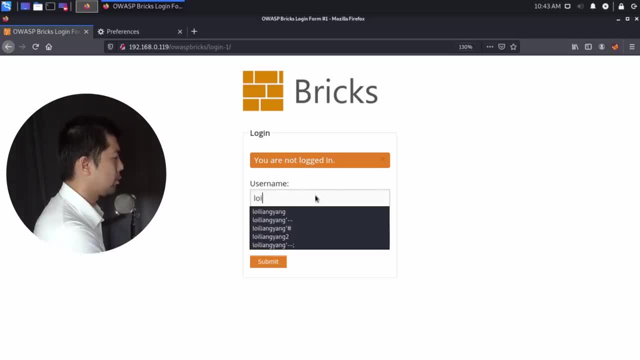 states that you are logged into the web application system. So if I go ahead and enter, say, for example, a username called Loy Leung Yang, and I enter some random password and click Submit, And of course, right here it states the following: Wrong username or password. And you see one more. 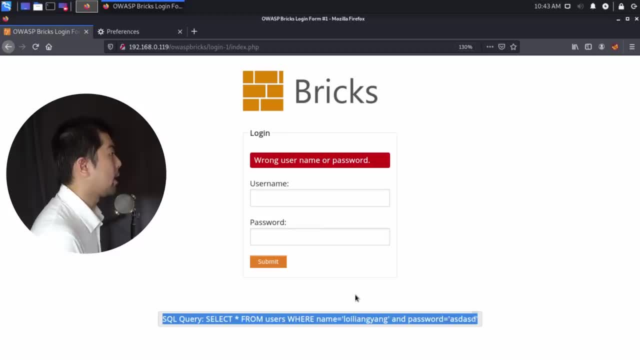 particular notification at the bottom, one message here, which is the feedback, And this is useful for you to picture what is going on behind the website as the application server tries to connect to the database and pull out query from the database system, And the database houses all. 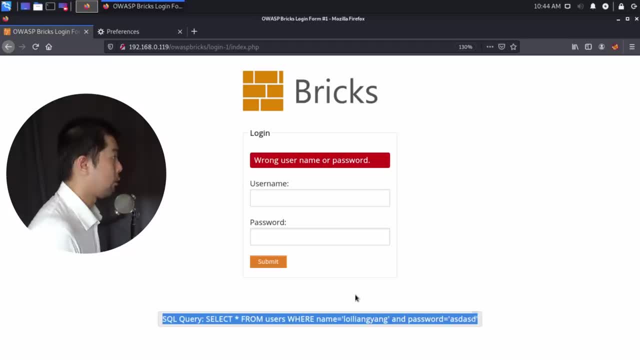 these records like usernames, passwords, email address and so on. So let's go ahead and click on it And you can see that it has a lot of personal and sensitive data. So, right here, what we can see is that we have the following. I'm going to copy this. I'm going to go ahead and open up, say, 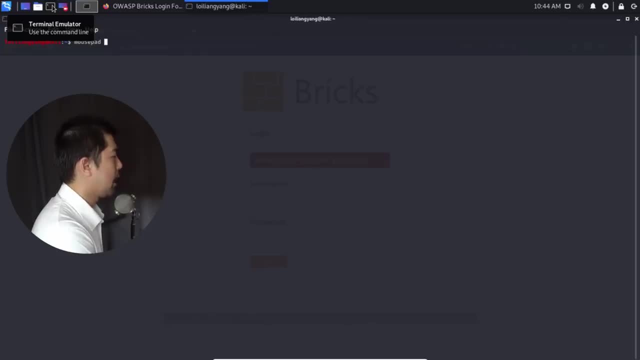 a text editor, And I will call it, say, I will use Mousepad, Okay, And we can go ahead and open it up, And I can do a right click and I can paste it right here And we can see over here And this is: 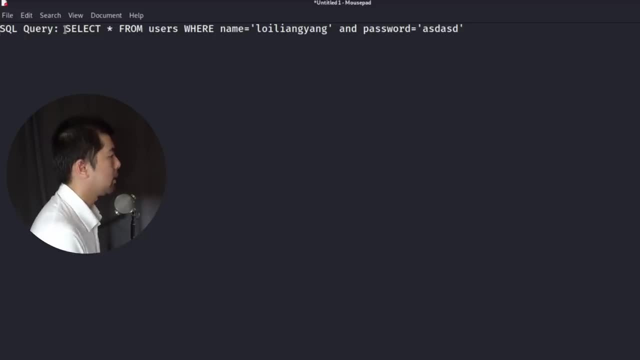 how the application service talk to the database, literally. So here we have select star, which is all from users where name equal- All right, Followed by name equal, And then we have the password, And this is the query that is being sent over from the application server into the 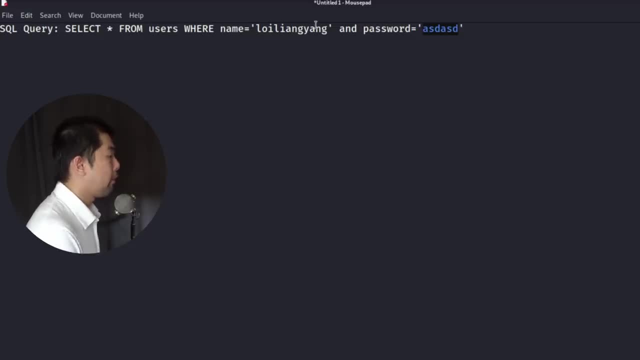 database And right here, what we can notice is that we are trying to find ways of bypassing the security mechanism And say we know what is the name. Perhaps that there is a username that we could find on LinkedIn as part of information gathering We could find on Facebook about the. 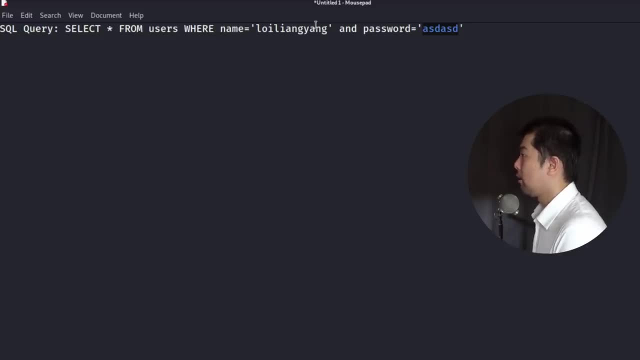 employees of the company, All right. Or even in the website itself, they could have a particular page that shows the employees who are working in the company As a directory, and so on. So many different ways to do a reconnaissance, to do information. 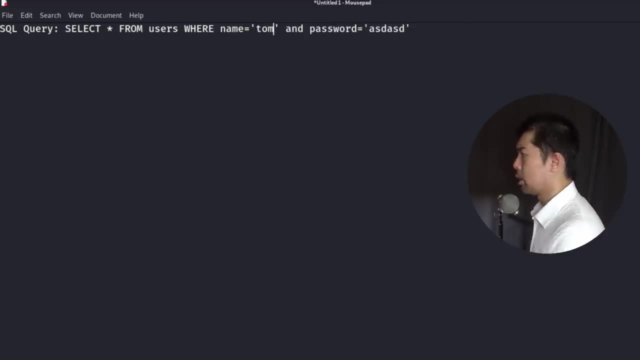 gathering. So here all you got to do is say: enter someone you know, So it could be Tom right. So in this case- and we have the password field, So what we can do- so in a SQL query, what we need to do is to ultimately get a true statement. So all I got to do now is to enter: 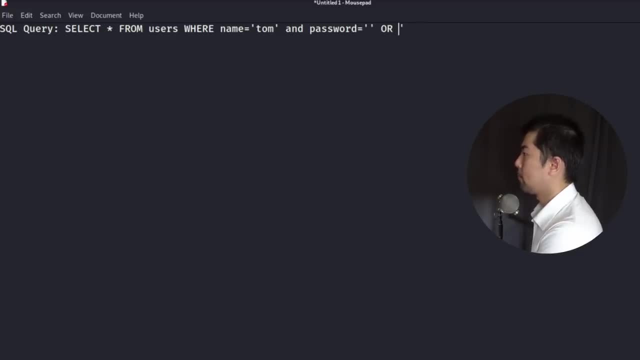 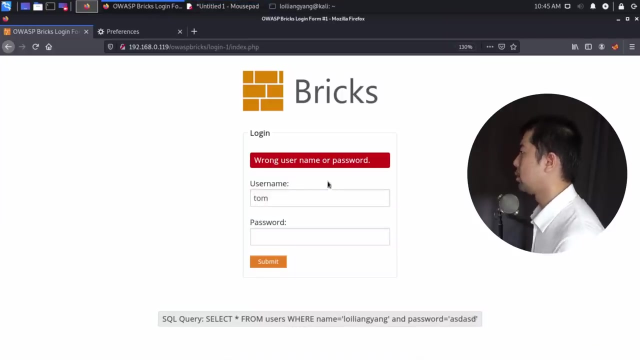 the following: Say: we have no idea what is the password We can enter, or, okay, one equal one, Okay, And let us try and insert this into the login page and look at what happens. So here I can go back into the website, I can enter Tom, And what I'll do next is to go. 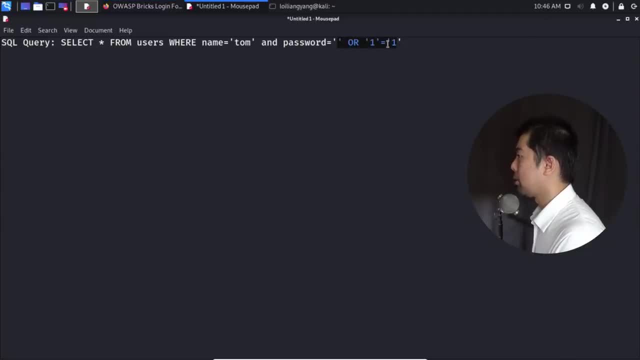 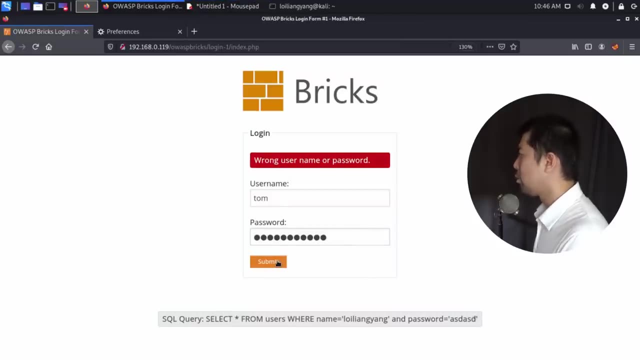 ahead and copy and paste the payload that we have just created right here. So I can go ahead and copy this and I'll paste it into the password field. So once I paste it, I'll click submit and let's see what happens. That's it. We have successfully logged into the site Successfully. 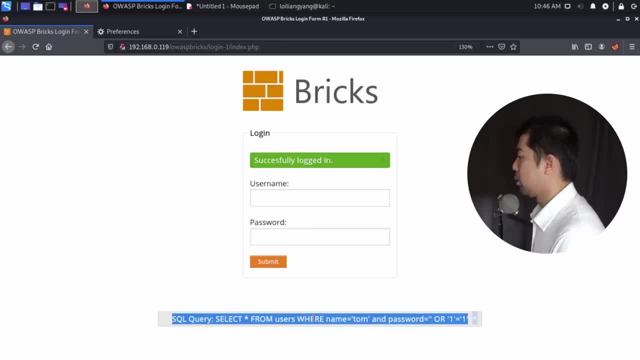 logged in And, as you see at the bottom, select all from users with name, equal Tom and password. okay is as such. or one equal one, Or one equal one means right. So if you remember back in school, one equal one is true and it. 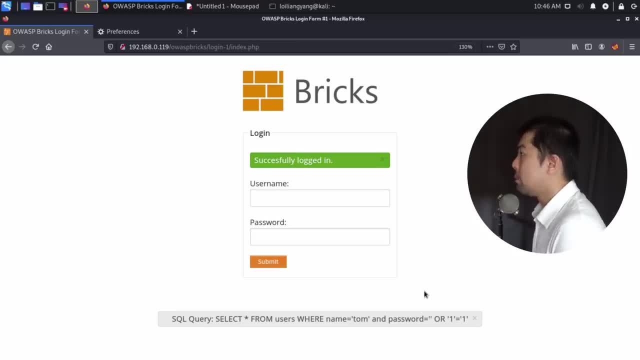 always is true, Or one equal one means that it will always be true. This statement is always true And, as such, as a result of that, the web application server will issue you, say, a cookie, a session cookie, whichever the case is, and you will gain access into the site- A lot of sites. 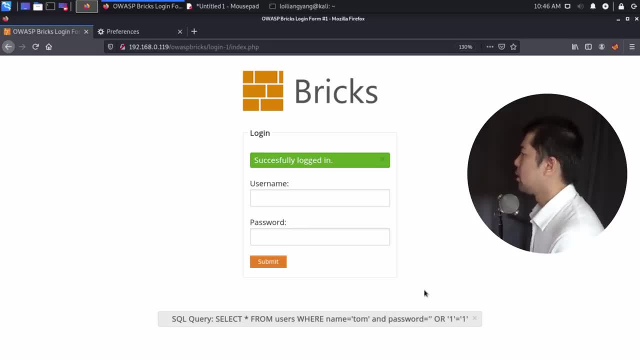 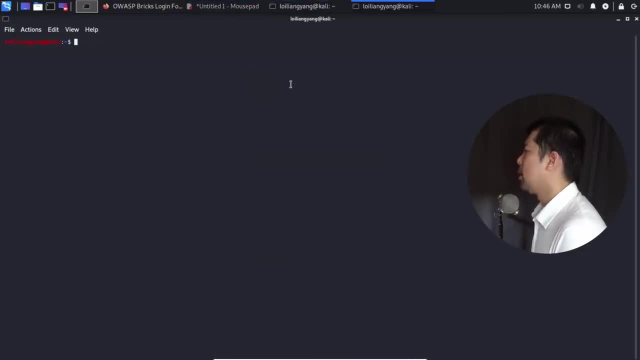 are pretty secure now and they would have different layers of security. So one of those particular word lists that you want to look out for is actually the word list that could help us find out whether, okay, we have different kind of payloads that we can utilize as part of the SQL injection. 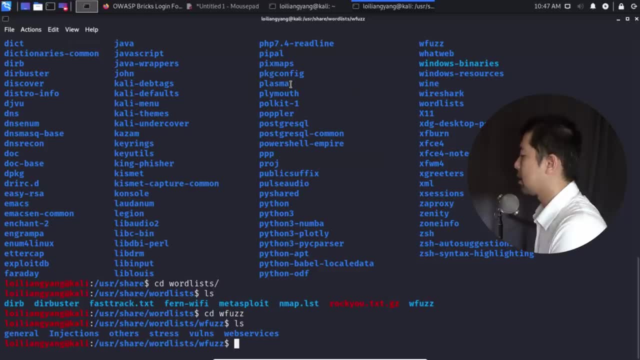 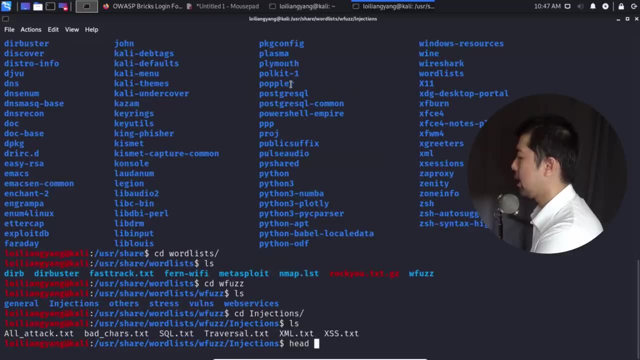 And we have over here. we have general injections, others stress vulnerabilities, web services. So let's go ahead and cd and change directory into injections, enter ls And I can do say, for example, hit sqltxt. So these are all the different kind of payloads that you can inject. 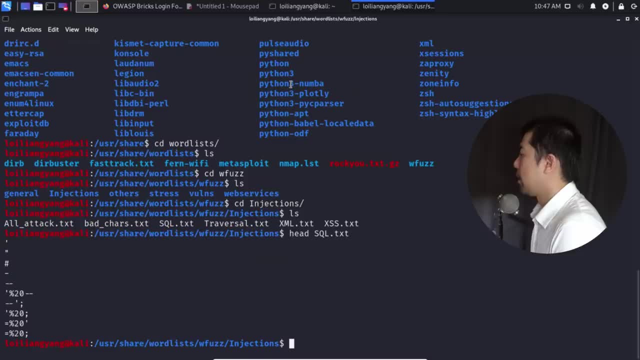 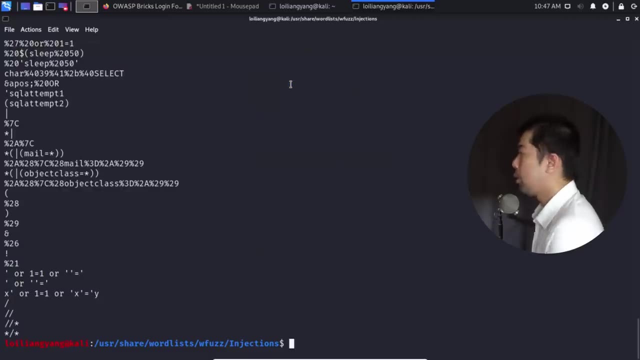 into the site literally, And this is how we can identify whether this particular input field is vulnerable to it. So I can enter cat sqltxt, hit enter on this. see all these different SQL payloads that you can inject into the page. Say, for example: 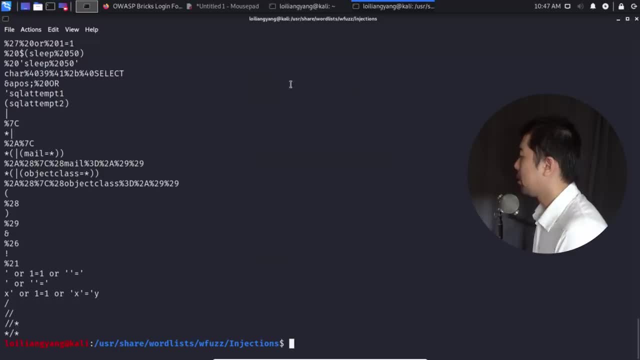 your single quote, your double quote didn't work. Then what can we do? What we can do now is to use other forms of payloads here that you can see, to run the attack against that specific parameter and see whether we're able to ultimately get an error page all right, or to get some kind of 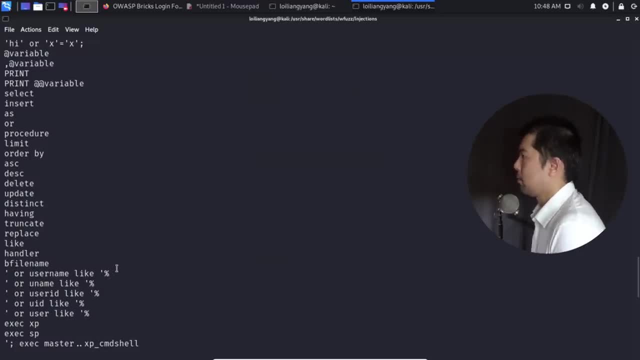 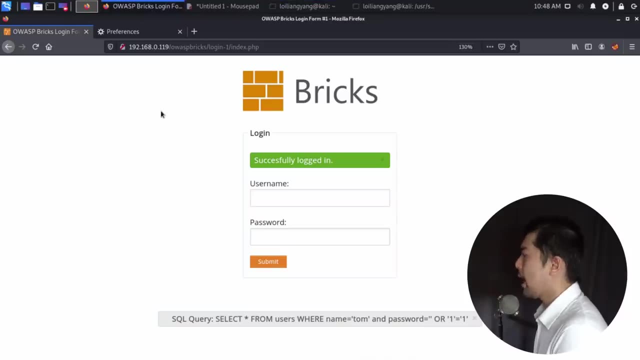 response from the server that is different from what is normal, And that's the whole idea behind SQL injection. And, next up, what I want to introduce to you is a way for us to do a highly automated matter in terms of finding out whether the input fields are vulnerable. 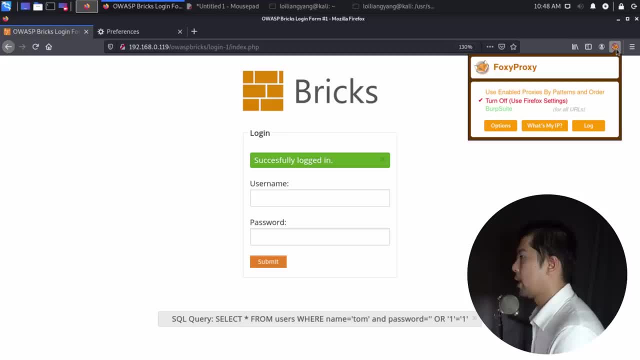 So what I can do now is go ahead and go to the top right corner. I can use Foxy Proxy and we'll click under Burp Suite. So this will enable the proxy to intercept our posts into the site. So all I got to do now is just go ahead and enter Burp Suite So I can launch Burp Suite directly. 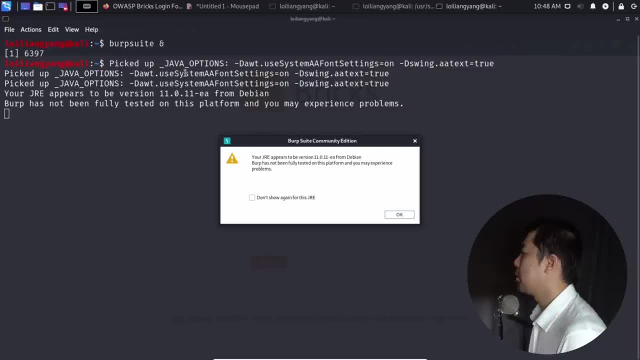 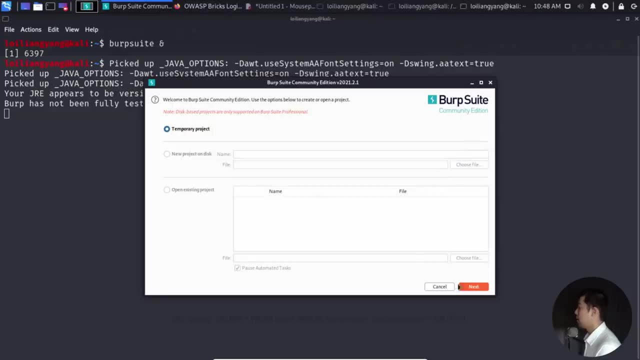 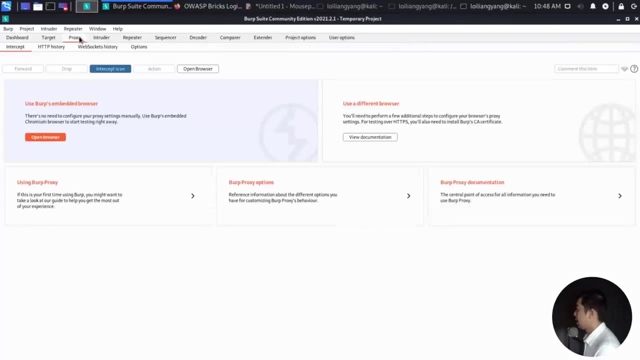 from here so that we can see what kind of post is being sent over into the site. okay, So here I can throw in temporary file. I will not update now. Click Next, Use Burp Defaults And right here we have the Burp Suite Community Edition And we click on the Proxy tab and ensure the intercept. 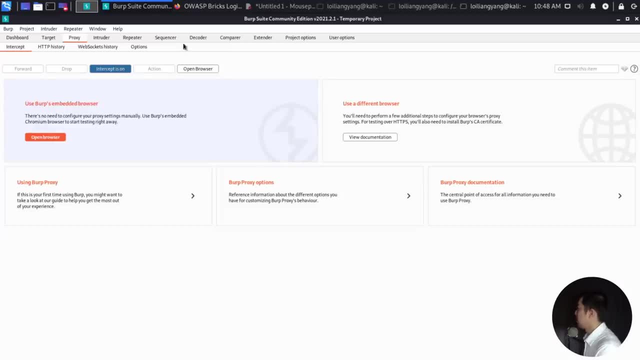 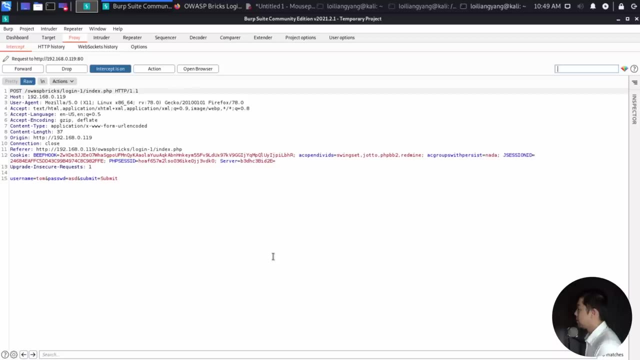 is on. So here we can see that intercept is on. So that's great. So what we can do next is to go ahead and enter some normal value and go ahead and click Submit, And that will get intercepted immediately by Burp Suite, as you can see right here. So what I can do now is to copy the entire. 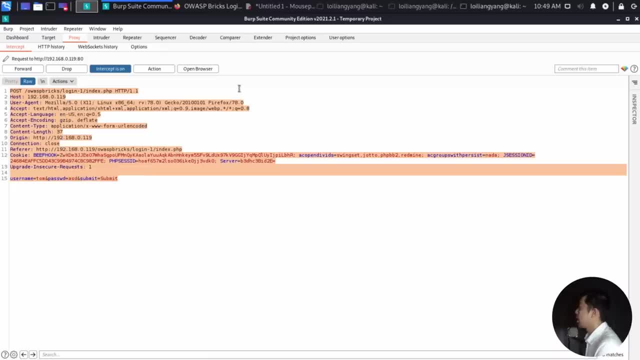 post. all right, the entire post, request and copy it, And what I will do now is to save it into a file. all right, So I'll save it into a file And I can go ahead and save this file. all right, So. 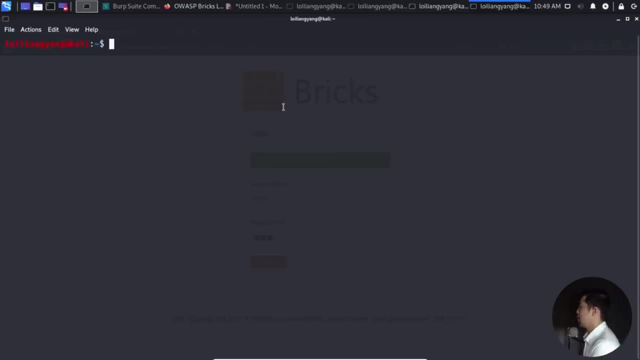 let's go ahead and say: create a file And let's name it as OWASP Bricks SQL Injection- okay. So let's go ahead and do a touch OWASP Bricks Injection- okay, Hit Enter on this And what I? 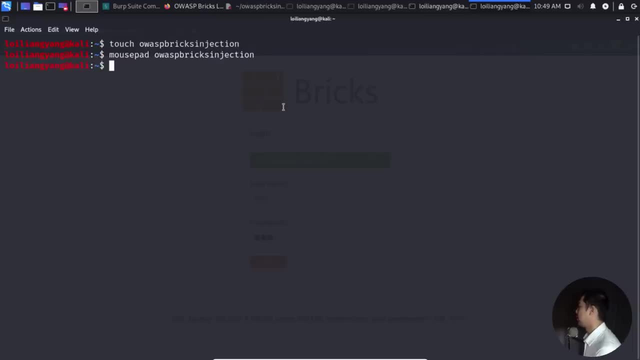 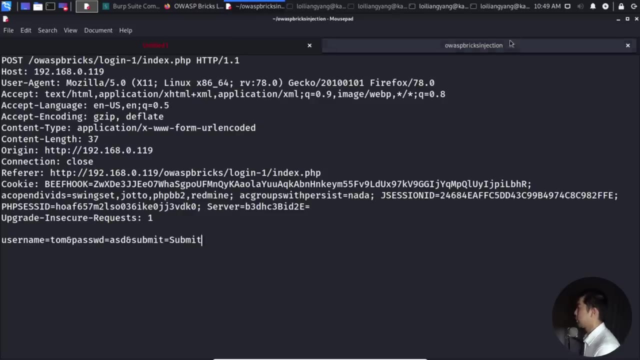 can do next is use a mouse pad, open up this particular file. all right, So open it up And we can see right here And I can paste it And I can save it. So let's go ahead and save the information. So this is OWASP Bricks Injection. okay, So what I can do next is to go ahead and 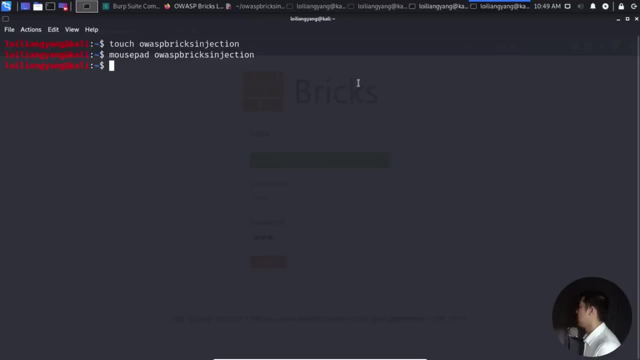 use SQL Map to help us target the parameter automatically to find out whether it is injectable, whether it is vulnerable to structured query language injection. So all I can do now is enter SQL Map: okay, followed by dash R to specify the file that we have just created, which is the. 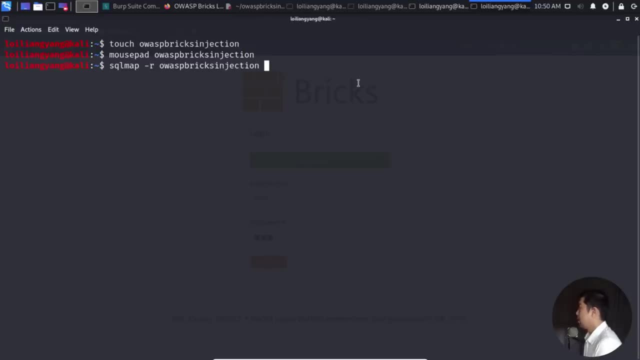 post request. So we have OWASP Bricks Injection, all right, And next what we can do is to specify the target parameter. So in this case, we can enter the following: all right. So we can enter the following: all right, So this is the parameter that we're going for. So enter username, So hit. 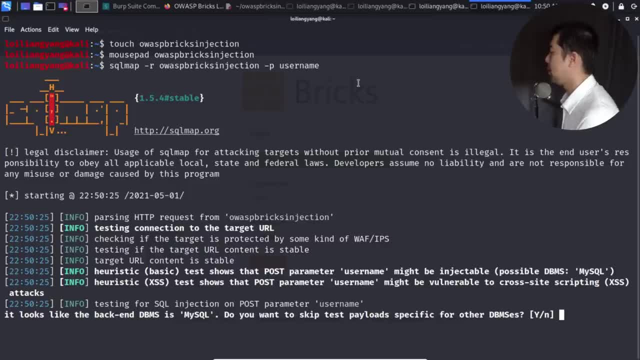 Enter on this And you can see right here. all right, It looks like the backend DBMS is MySQL. Do you want to skip task payloads specific for other database management systems. So very, very quickly we are able to identify vulnerable parameters. So, as you can see here, username might. 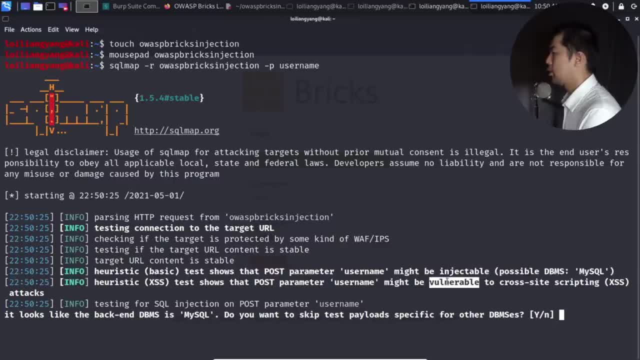 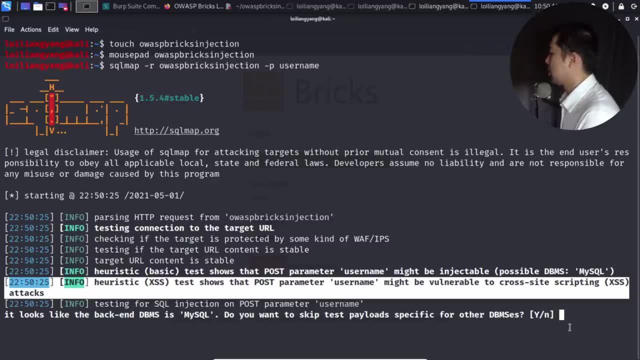 be injectable. So that's one MySQL database, And two might be also vulnerable to cross-site scripting, which we will do up on a separate tutorial. So do we want to skip? Yes, So it could save us a lot of time. And do you want to include? 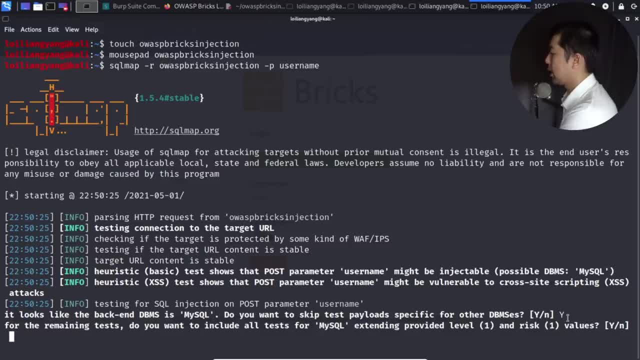 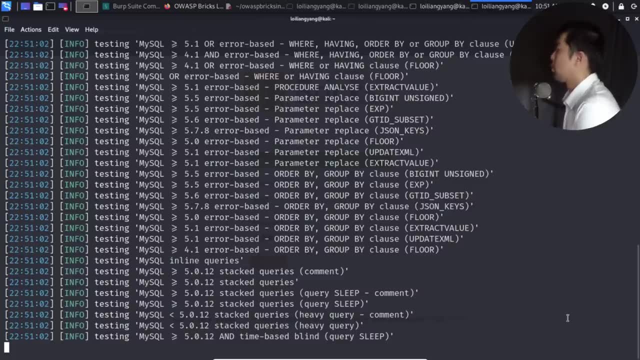 all right. all tasks for MySQL extending provider level. All right. so let's go ahead and enter yes for this, And right here it is running all those injections into this particular parameter to see whether we're able to probe the database, whether we are able to bypass the web application checks. 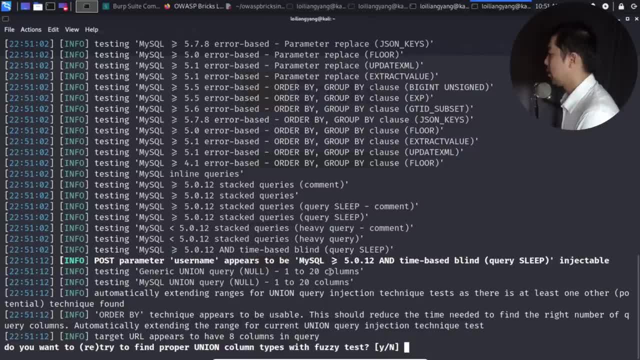 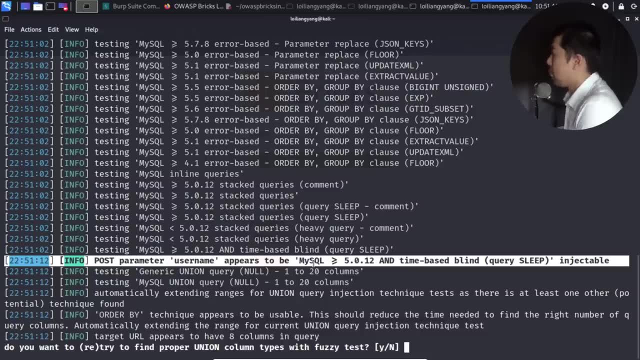 the sanitization, And very quickly. right here we can see that the following time-based blind is injectable, Meaning that we have found a way for us to bypass the security checks and gain full control of the database. Just like that. very, very quickly we are able to identify the vulnerable parameter. 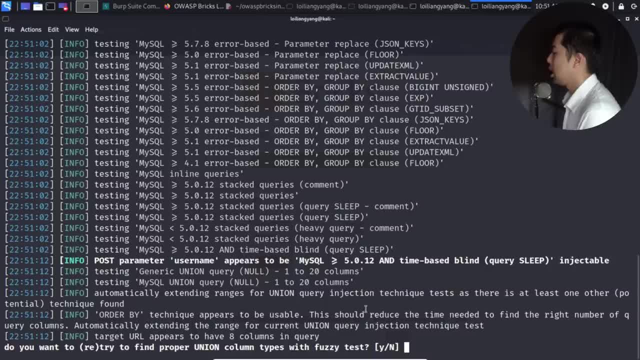 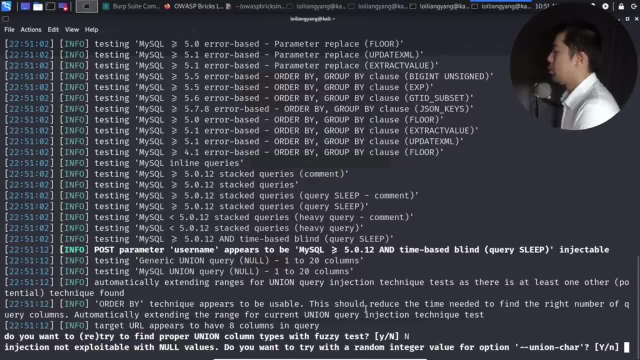 And what we can do next is the following: Do you want to retry to find proper union column types with fuzzy tests? So enter no for this. Okay. injection not exploitable with null values. Do you want to try the random integer value for option union corrector? All right, so enter yes. 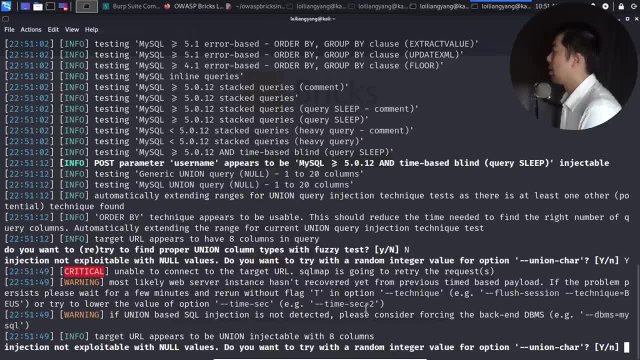